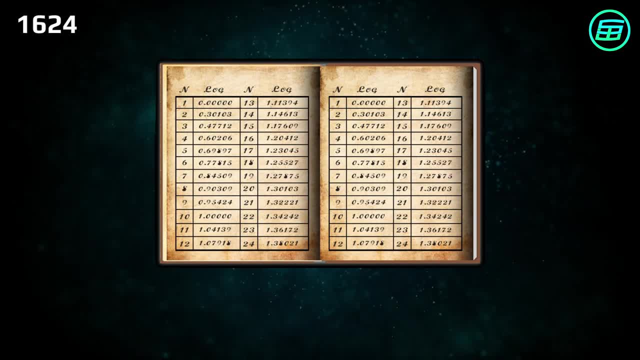 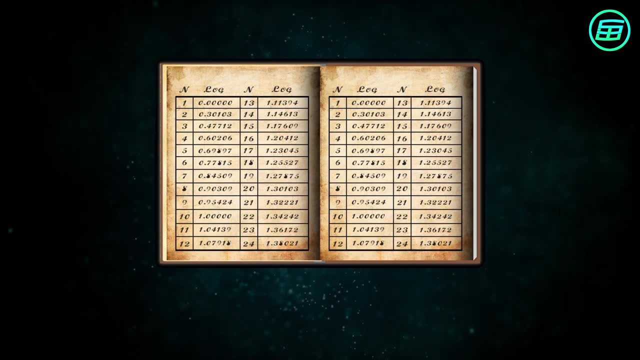 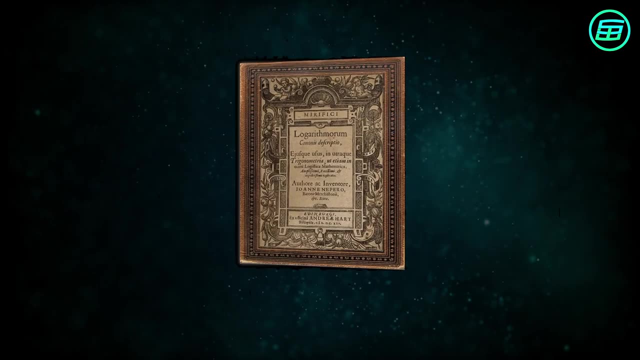 other scientists extended the list By 1624. the list included the logarithms of all the numbers from one to a hundred thousand. Using it, people could quickly find the logarithms of two or more numbers and convert multiplication operations into additions. For example, suppose you bought 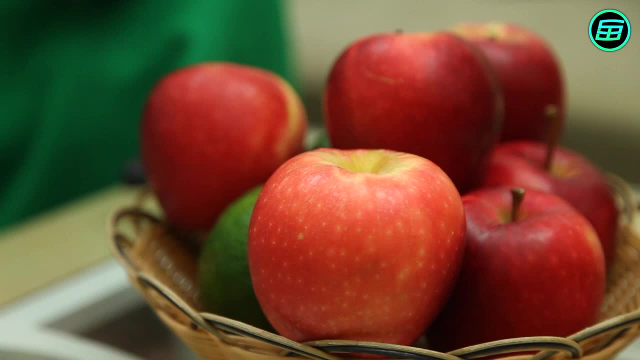 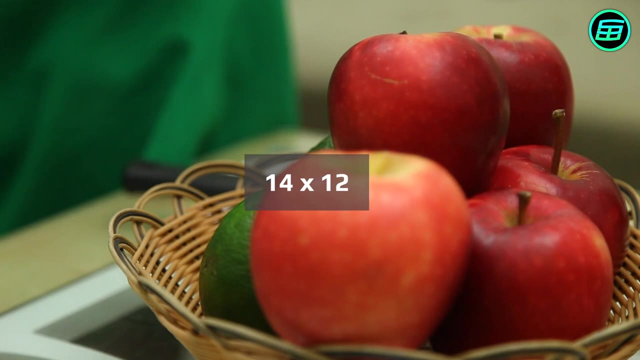 14 apples from a market and each apple costs 12 cents. The amount you'd have to pay is 14 times 12.. Using Napier's method, first we need to find the logarithm of 14 from the logarithm list. It turns: 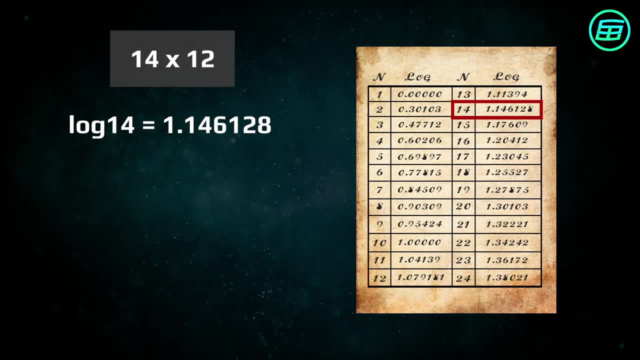 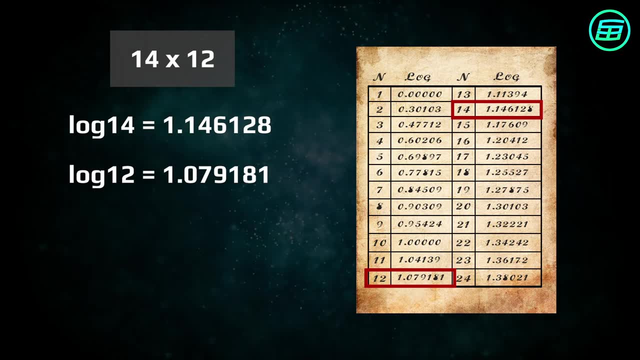 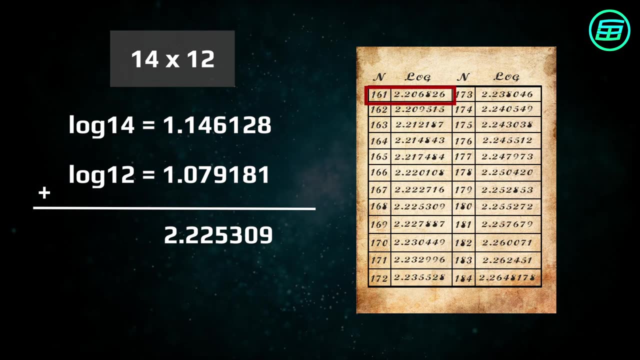 out to be 1.146128.. Then we need the logarithm, or log 12.. It's 1.079181.. We add these to get 2.225309.. Finally, we look at which number from the list corresponds to this log and find our answer: 168.. 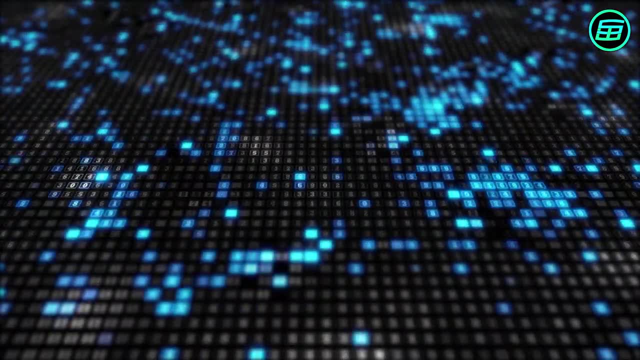 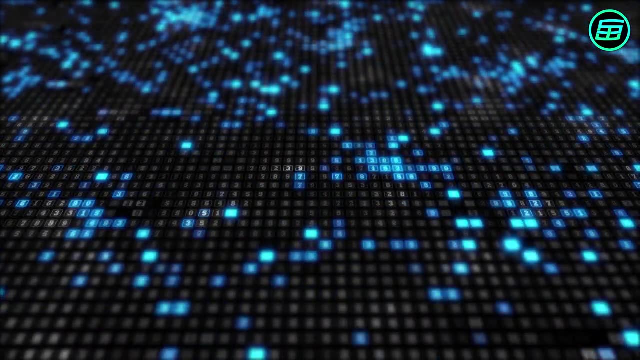 When we add 2 to our total, there are a total of 7.1.. In this simple case, it's true that it's quicker just to do the multiplication, but the advantage of logarithms becomes clear when we start dealing with more numbers or bigger numbers. 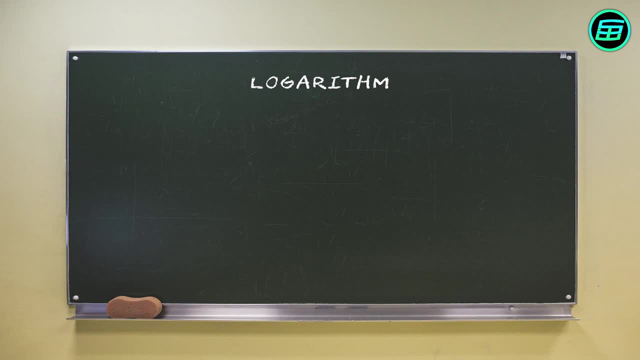 In mathematics, logarithms is the process used to find exponents. For example, what's the power of 2 that gives 8?? The answer is 3.. 2 is 3.. A common base to use is 10,, in which case we have the following: 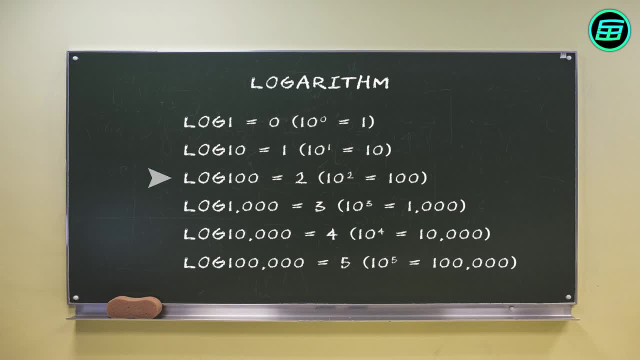 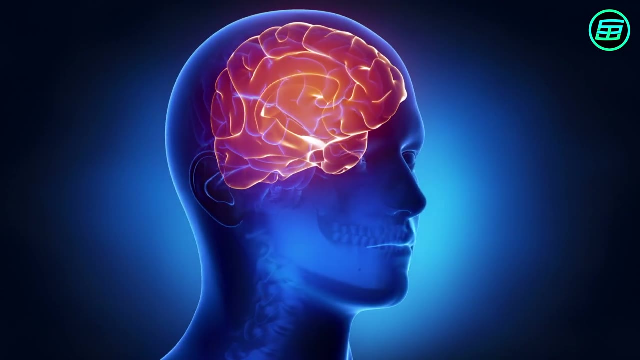 Log to base: 10 of 100 is 2 because 100 is 10. squared Log 10,000 is 4 because 10,000 is 10 to the 4.. Often our brains perceive changes in the environment not linearly but logarithmically. 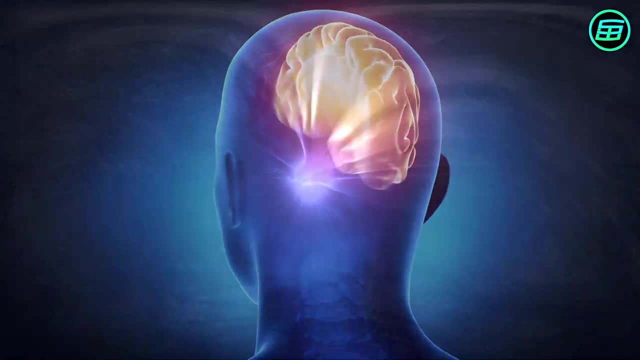 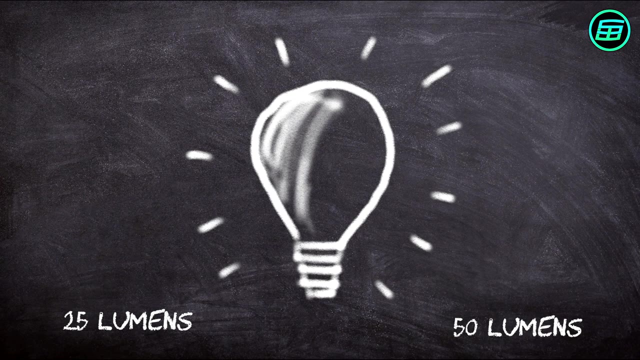 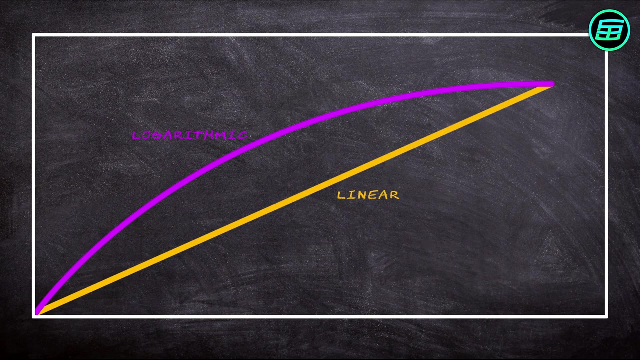 For example, when we compare two light bulbs that have intensities of 25 and 50 lumens, we don't perceive the intensity of the 50 lumen bulb to be twice as great as that of the 25 lumen bulb, but much more than that, In fact a logarithmic increase. The same is true of our 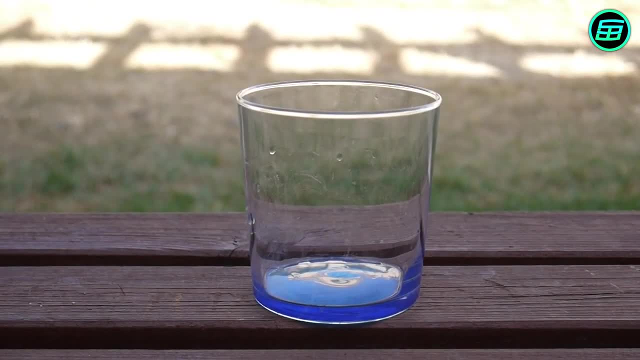 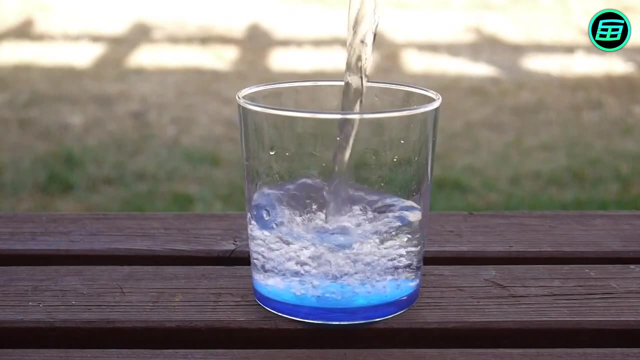 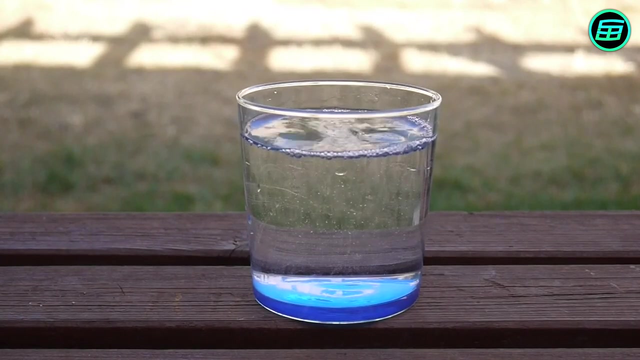 sense of taste When we compare the same amount of water with 50 and 100 grams of dissolved salt. after taking a sip of each, the water containing 100 grams of salt is perceived as being much more than twice as salty as the water containing 50 grams of salt. Research also suggests the same. 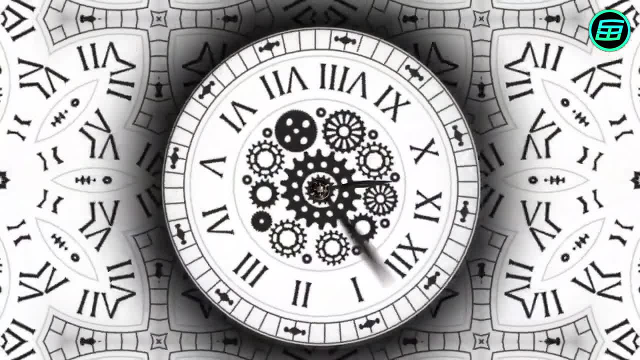 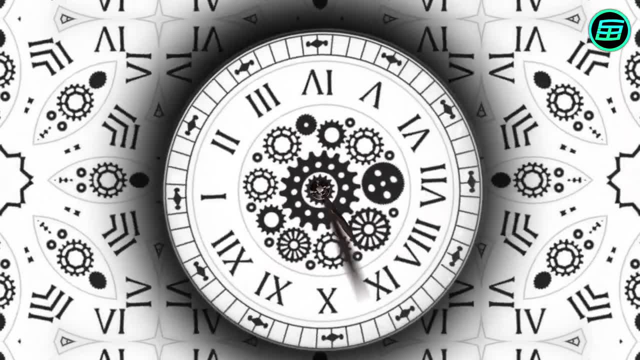 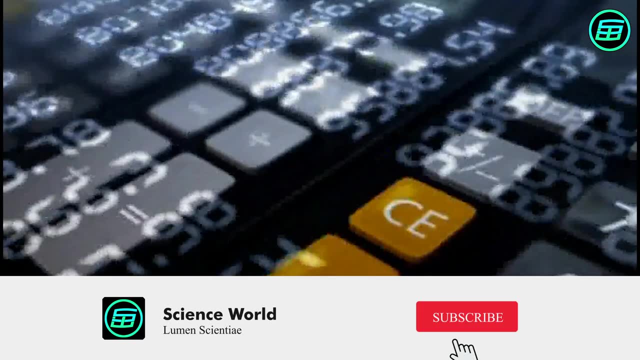 is true of our perception of time. As we get older, time seems to go by much faster. A 10 year old and a 70 year old, for instance, perceive the passage of a one year period very differently. In practical applications, logs are used mostly to deal with very large or very small numbers. 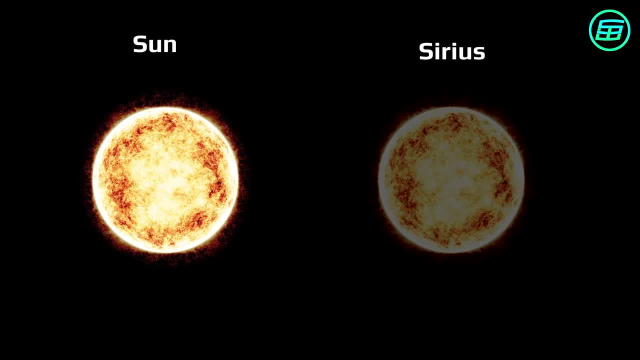 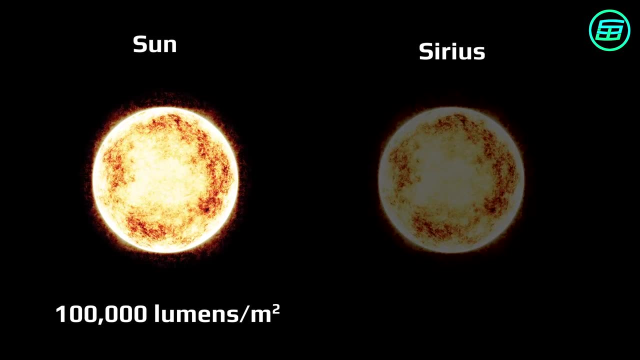 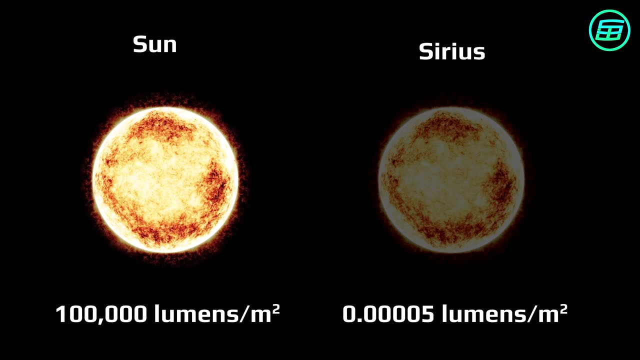 The brightness of the sun, for instance, is about 100,000 lumens per square meter, whereas the brightest star visible at night has a brightness of 0.00005 lumens per square meter. It's hard to grasp such big differences in values, but if we switch to a log scale, 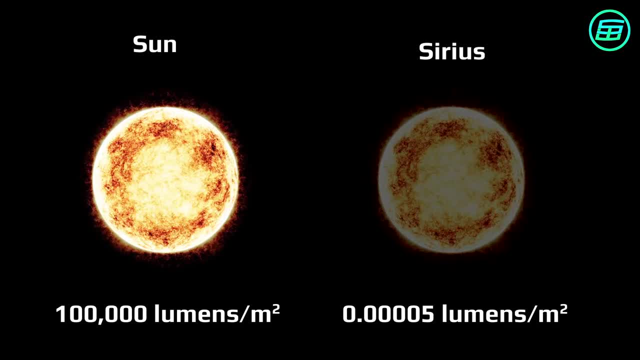 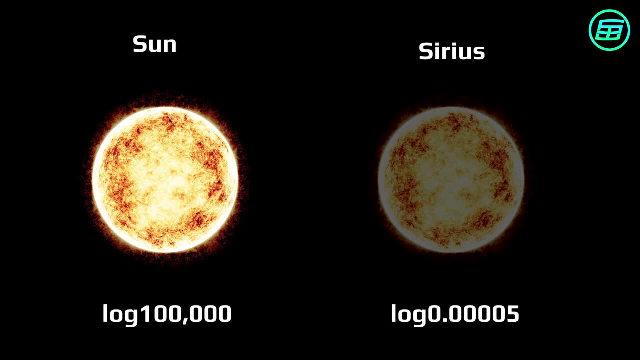 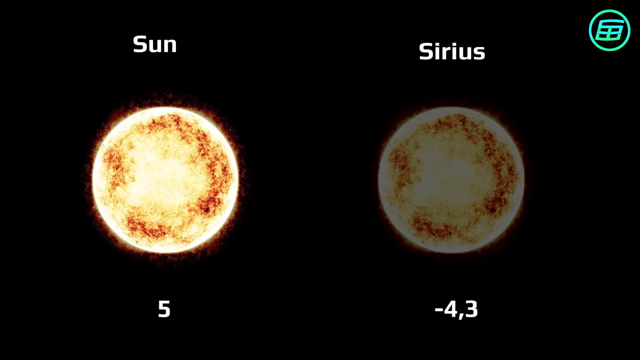 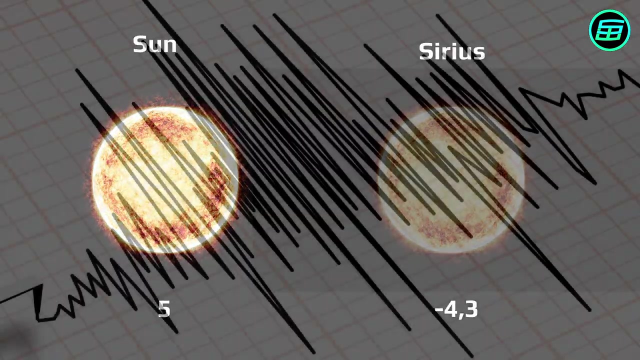 the numbers become much more manageable. The brightness of the sun becomes log 100,000, which is 5,, and the brightness of Sirius, the brightest star at night, is log 0.00005, or minus 4.3.. Let's take a look at some other examples of logarithms in real science. As you know, 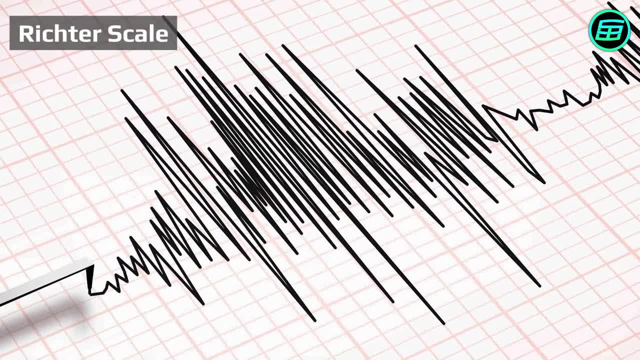 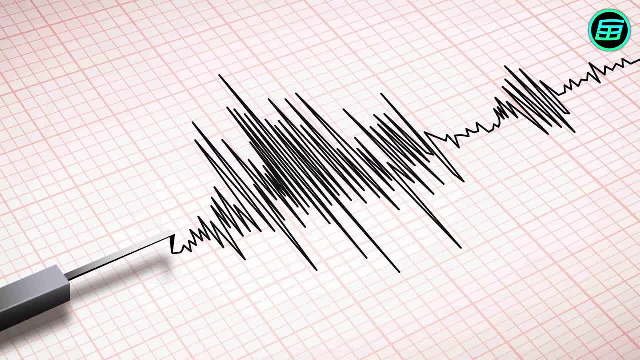 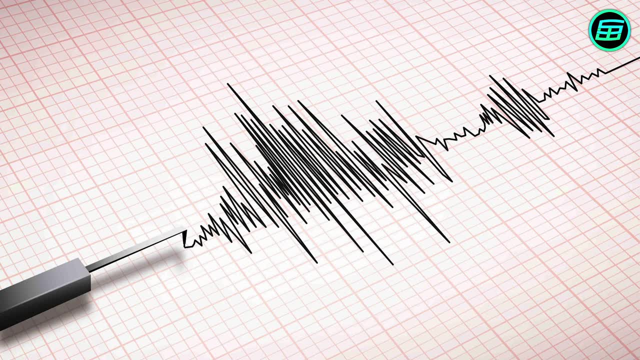 the Richter scale is used to measure the severity of earthquakes, And it's a logarithmic scale, so an earthquake that measures 6 on the Richter scale isn't twice as severe as one that measures 3 on the Richter scale, but 1000 times more powerful. 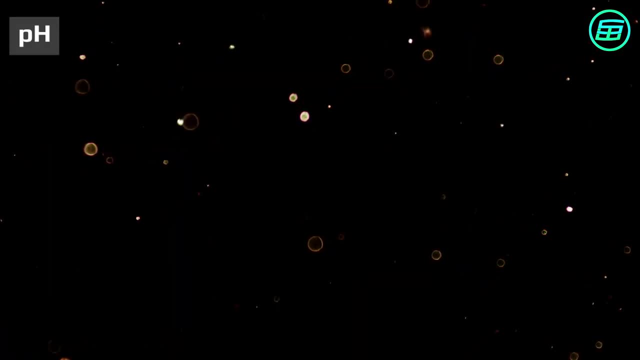 For a substance to be an acid, it must give positively charged hydrogen ions to its environment. In the term pH, H represents these ions, while the letter P is a mathematical function that denotes minus the logarithm. So pH is the negative log of the hydrogen ion concentration. For example, the pH value of water is about 7,.